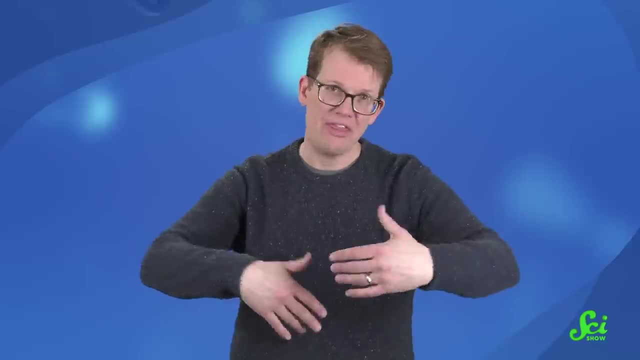 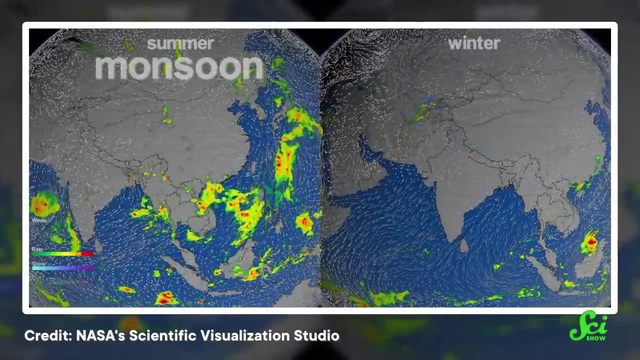 cool ocean air rushes in to take its place. There you go. that's where wind comes from, And in the case of summer monsoons, ocean air also brings a bunch of water vapor with it and several months of rain. When September rolls around, the temperature difference between the land and sea evens. out and the rain stops, But by December the situation has flip-flopped. The continent turns chilly, but the ocean still maintains a little of that summer heat, and the winds shift seaward. Now these dry monsoons don't look like very exciting weather from the perspective. 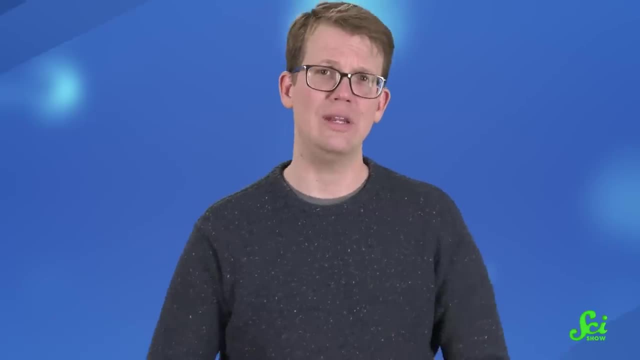 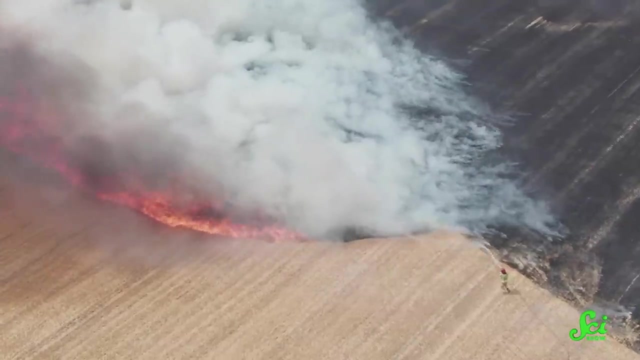 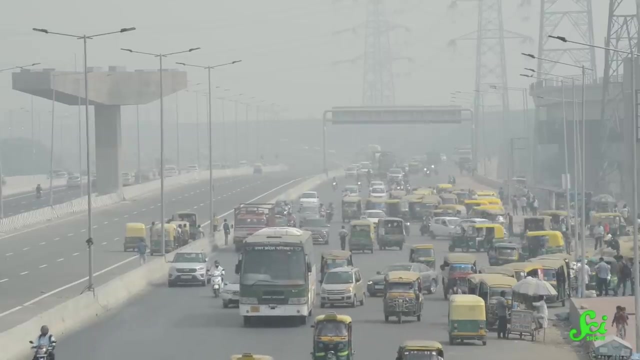 of someone living in Mumbai or Bangkok — they're just a long string of windy days, But they have a super-important job worldwide: They carry away pollutants. When humans create a bunch of air pollution — say by burning crops, running industrial factories or driving gas-powered cars — it often forms an atmospheric haze that just 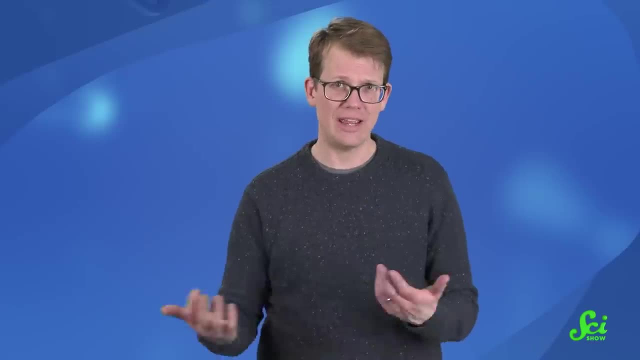 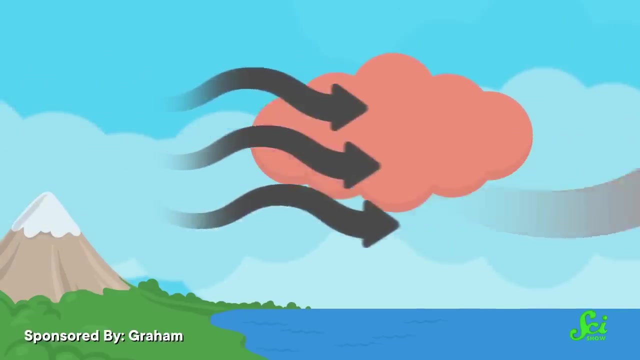 hangs out over whatever land it came from. Not so nice to breathe day in and day out, but nature has a way of cleaning it up. When the winter monsoon winds show up, they carry pollutants like carbon monoxide and lead in the air. 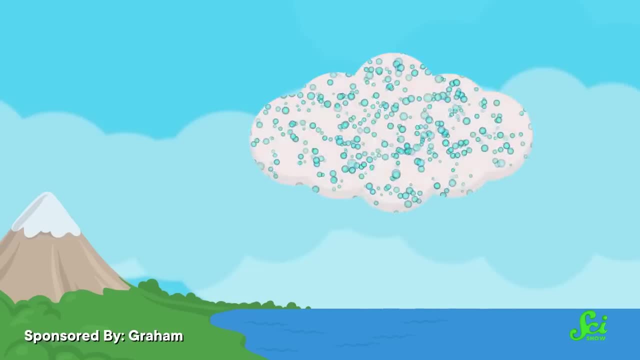 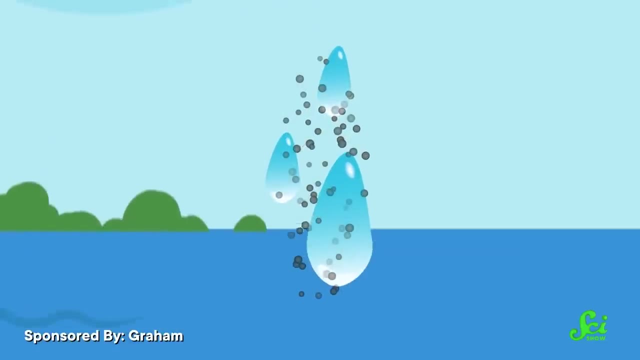 They're out to the ocean. Once it's there, the dry air can pick up some moisture, And since a single raindrop can attract dozens or even hundreds of aerosolized particles as it plummets through the air, these pollutants can sink to the bottom of the ocean whenever. 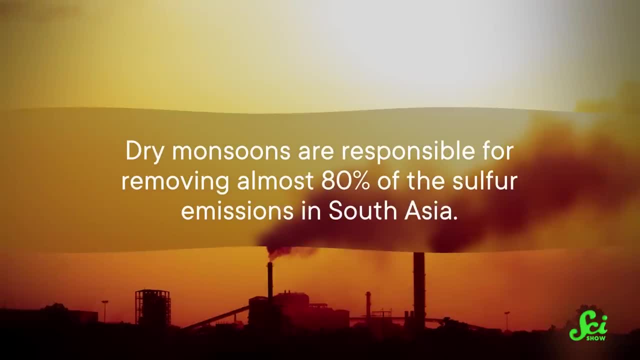 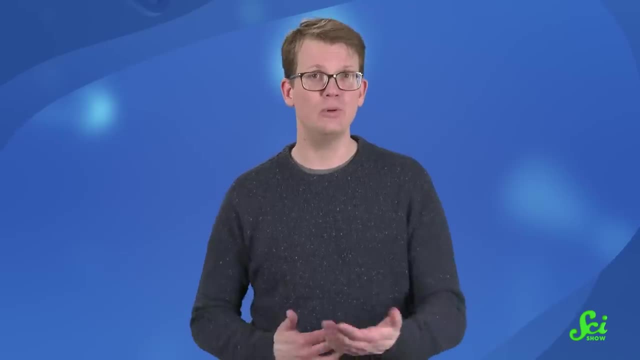 it rains. Back in 2018, researchers reported that dry monsoons are responsible for removing almost 80% of the sulfur emissions in South Asia. Sulfur is dangerous because it's prone to react with other compounds in the atmosphere, resulting in pollutants like sulfur dioxide and even acid rain. 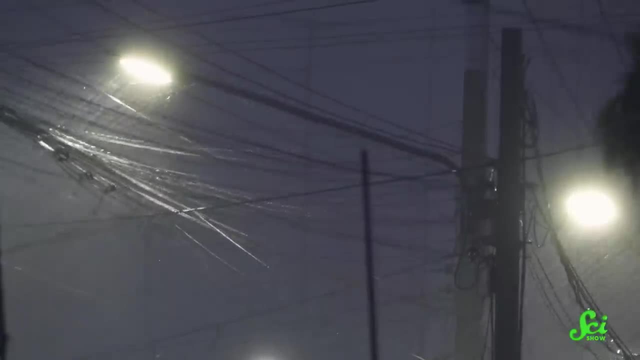 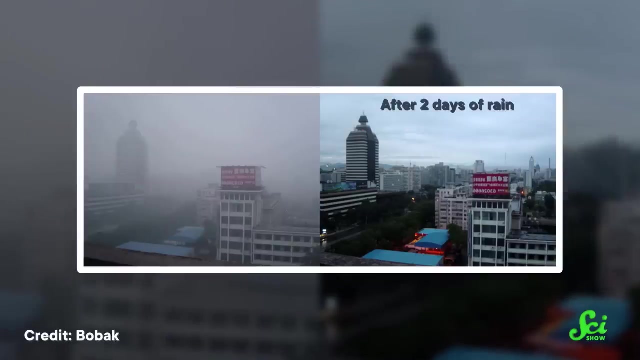 But dry monsoons shouldn't get all the praise. With their torrential rainstorms, wet monsoons can get it on the pollution-busting action too, Using the same process that dry monsoons do. once the air reaches the ocean, wet monsoons. 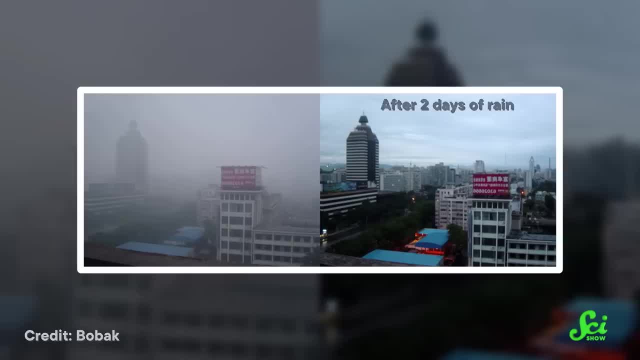 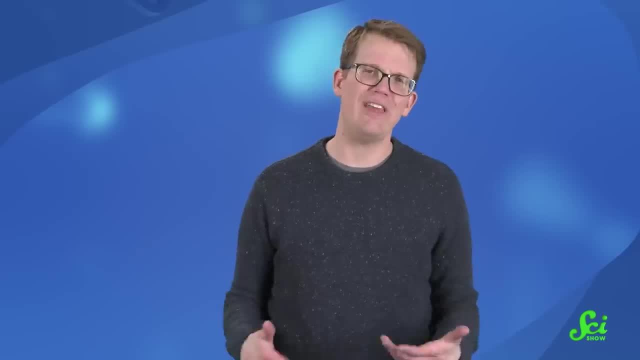 gather pollutants into the air and send them into the ground. So it's actually great news for humans and ecosystems that both wet and dry monsoons can clear out some of humanity's mess, But unfortunately they're not perfect air scrubbers. The same researchers also found that some pollutants extracted by winter winds aren't. snatched by raindrops and carried to the ocean's water, But they're not perfect air scrubbers. The same researchers also found that some pollutants extracted by winter winds aren't snatched by raindrops and carried to the ocean's water, But they're not perfect air scrubbers. The same researchers also found that some pollutants extracted by winter winds aren't snatched by raindrops and carried to the ocean's water. 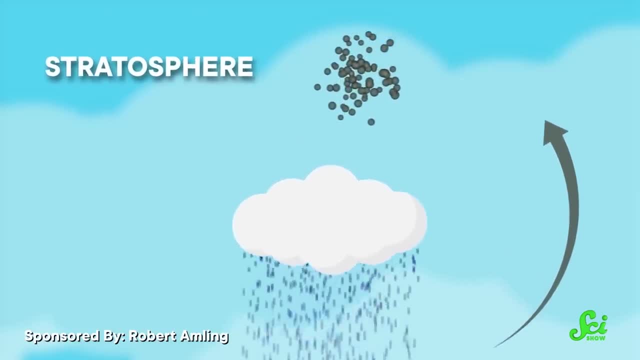 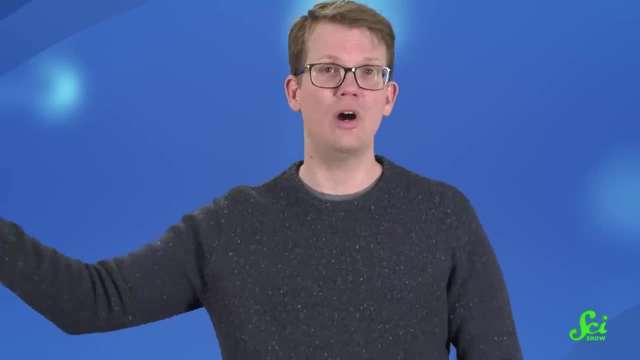 Instead, they're pushed up above the monsoon clouds into the stratosphere, the part of our atmosphere where the ozone layer lives. The ozone layer is great because it blocks most of the sun's harmful ultraviolet light from reaching living things down here. 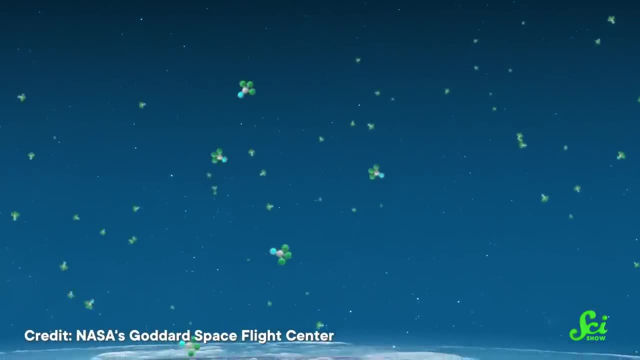 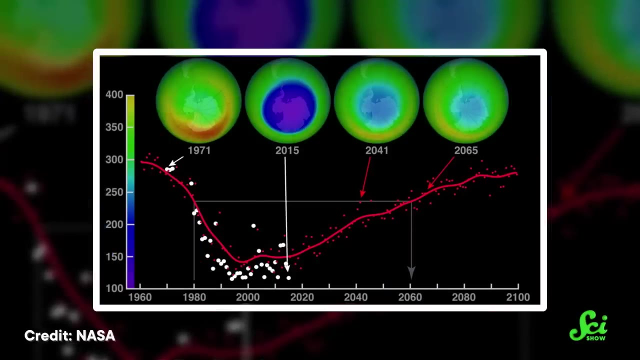 We love that ozone layer, But when pollutants get up there they can react with the ozone molecules and break them down, especially over Earth's poles. If all this sounds familiar, it should. We've worried about the thinning of the ozone layer before, but thanks to an international 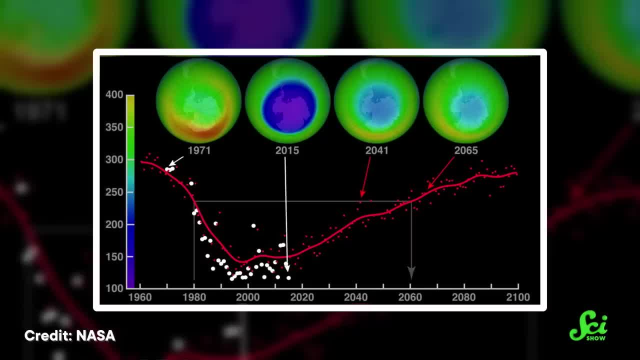 treaty passed in 1936, it's not a problem. But thanks to an international treaty passed in 1987 banning the use of some ozone-depleting chemicals, we've managed to reverse the trend. It would be a shame to see all of that hard work be undone. 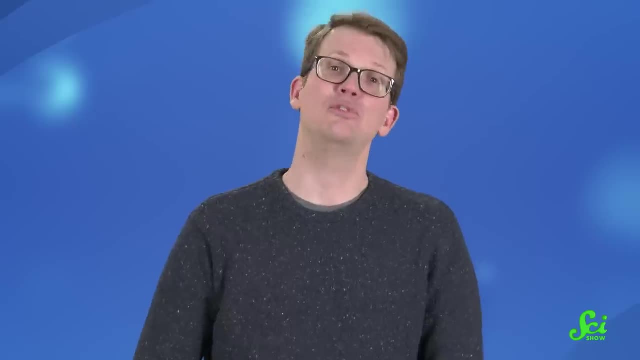 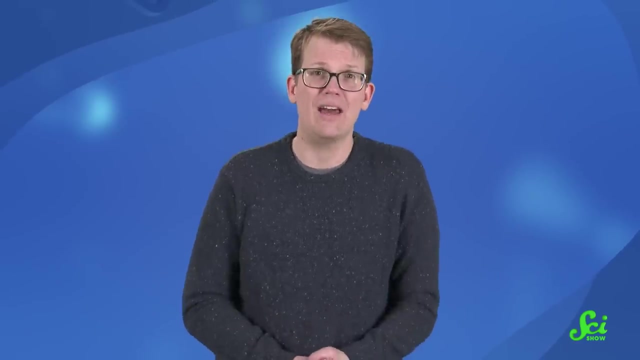 So we can't just keep letting pollutants leak into the atmosphere, assuming that monsoons will do all the hard work for us. Scientists are still learning about this ozone piece of the monsoon puzzle, although they might not have much time Due to warming temperatures on Earth. the rock-steady pattern of our planet's monsoon. 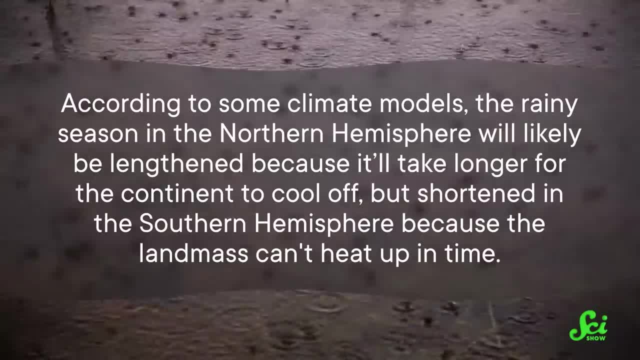 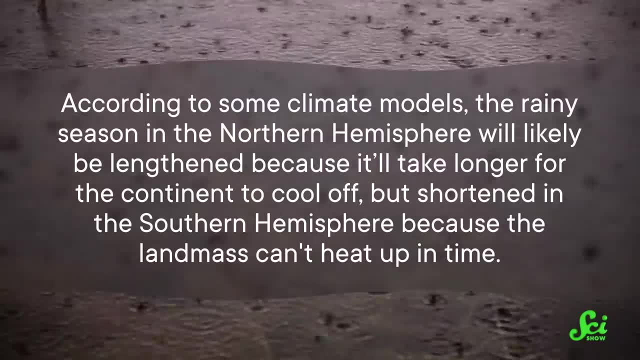 seasons is changing rapidly. For example, according to some climate models, the rainy season in the Northern Hemisphere is the worst in the world. The weather will likely be lengthened because it'll take longer for the continent to cool off, but shortened in the Southern Hemisphere because the landmass can't heat up in time. 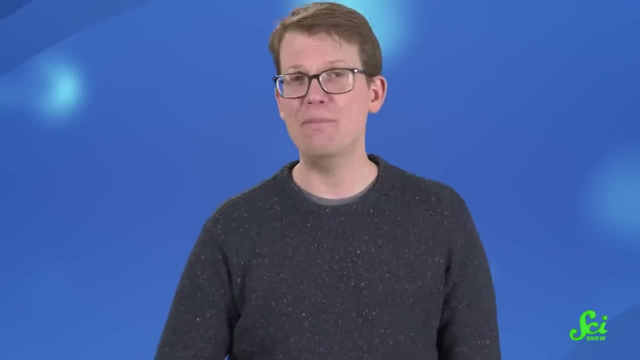 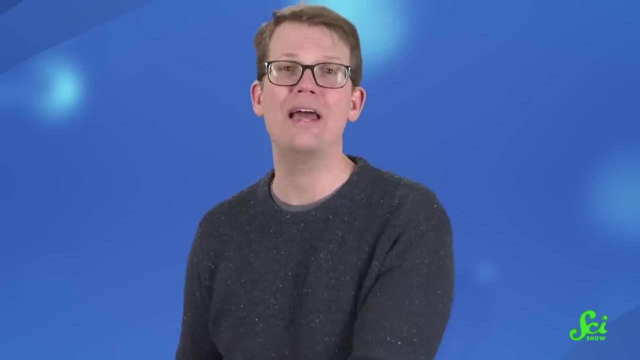 The wet and dry monsoon cycle has been running like clockwork for millions of years. If that gets thrown out of whack, it could affect their ability to carry our atmospheric trash to places where it can do less harm. While we may not fully understand the implications of the changing pattern, it's a critical 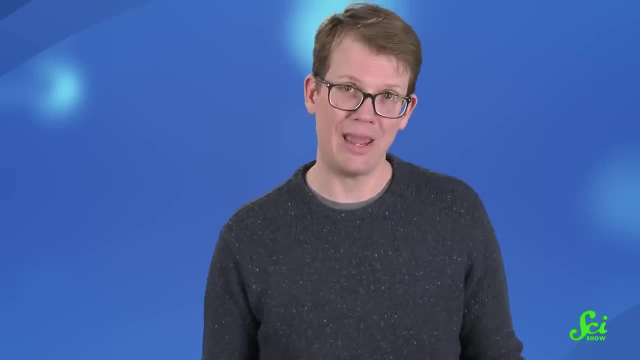 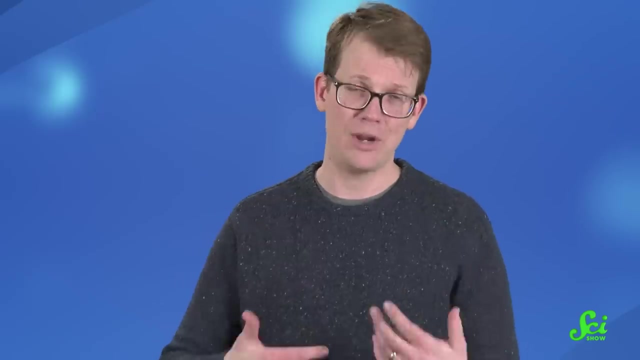 area of study for environmental scientists. Our future may depend on knowing which way the wind blows. With a somewhat unpredictable future, it always helps to have each other's support, And that is why we are so appreciative of the support we receive from our patrons. on 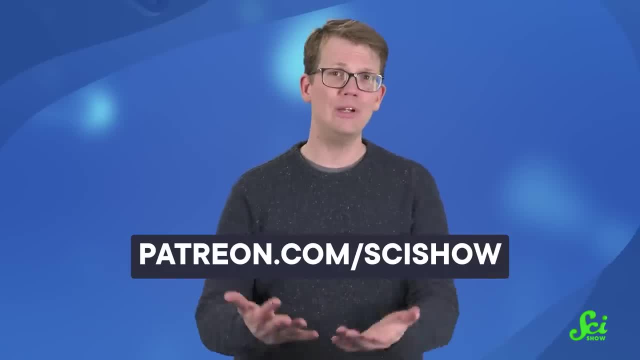 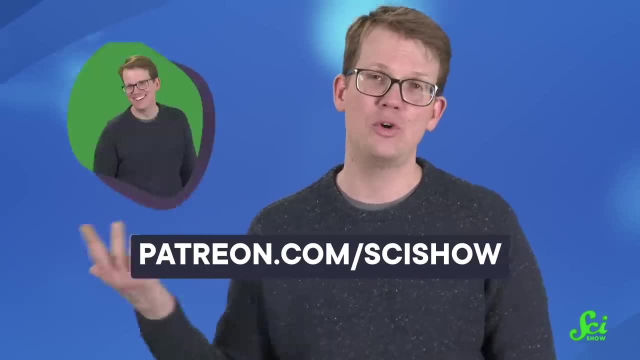 patreoncom slash scishow. By supporting SciShow on Patreon, you're helping ensure that your future is full of the videos that you enjoy. Plus, you get all sorts of perks, like bloopers, from these shows. We just recorded a video about hemipenes that's going to have a bunch of them. 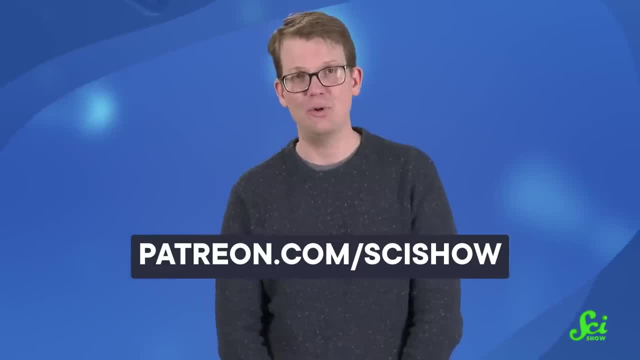 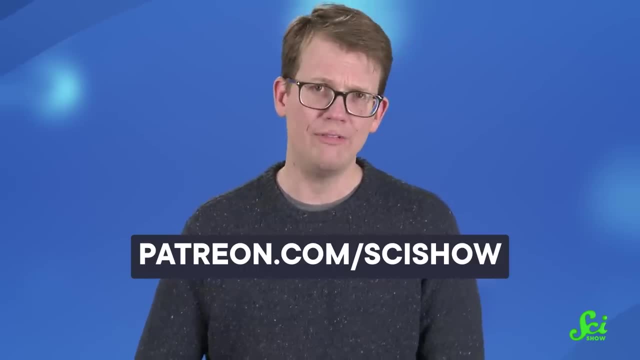 There's also our exclusive monthly podcast and access to the official SciShow Discord. To join the Patreon community, head to patreoncom slash scishow or click the link down in the description. We could not do all of this without you.